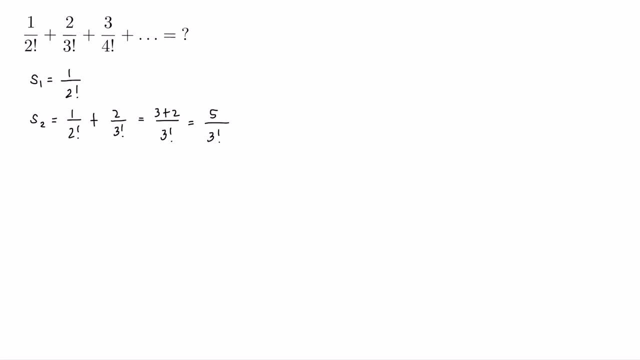 So this is equal to 5 over 3 factorial. And if we look at the sum of the three terms- first three terms- then that is equal to the sum of the first two terms, and then plus the third term, 3 over 4 factorial, which is equal to 4 factorial. So this is equal to 4 times 5,. 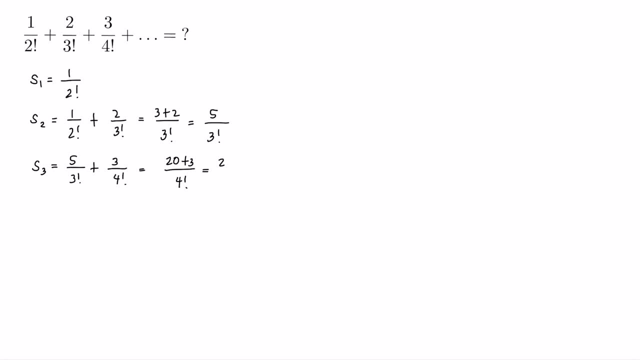 so that is equal to 3 over 3 factorial. So if we look at the sum of the first three terms, 20 and then plus 3, which is equal to 23 over 4 factorial, and from this we can already see a pattern, okay for this nth partial sum, because this 23 is actually 4 factorial minus 1, and this 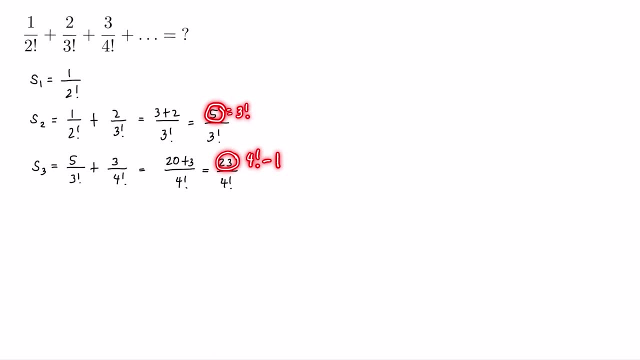 5 here is equal to 3 factorial minus 1, and of course this 1 is also equal to 2 factorial minus 1. so our guess in this case is that the sum of the first n terms, so s of n, is equal to, so the 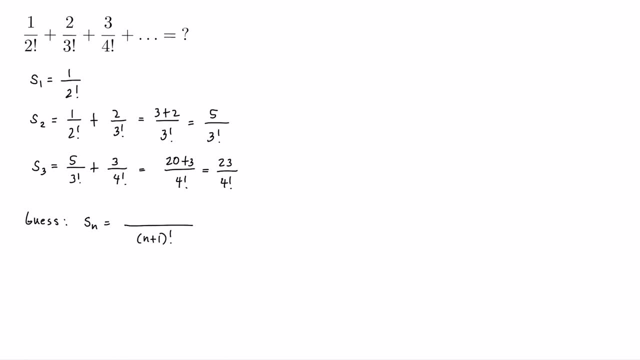 denominator is n plus 1 factorial and the numerator is just 1 less than this denominator, so n plus 1 factorial. but let us show that this is true for n element of the set of natural numbers. so to prove this, so let's do mathematical induction so clearly: s of 1 is equal to 2 factorial minus 1 over 2 factorial. 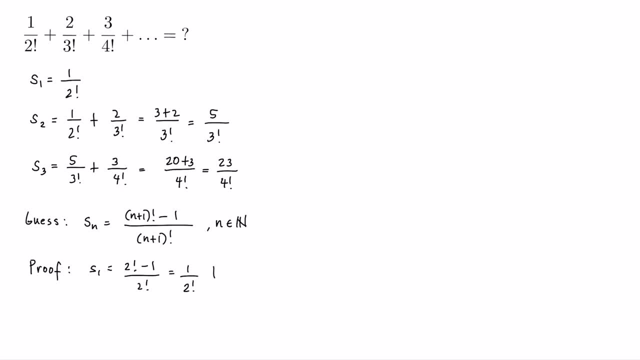 which is equal to 1 over 2 factorial. so therefore our equation is true for n equals 1. so now let's name this equation equation star, and then let's assume that star is true for n equals k. we're going to compute the formula for the sum of the subussia 1 and eThat is, s sub k is: 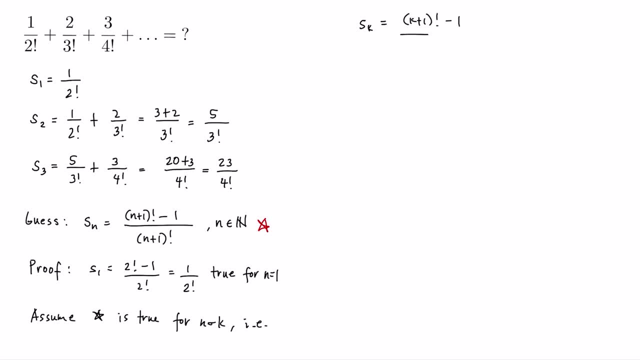 equal to, in that case, k plus 1 factorial minus 1, all over k plus 1 factorial, and we're going to show that it is also true for n equal to k plus one. but if this is true for n equals k, then in this case, if we're going to compute for the sum of the 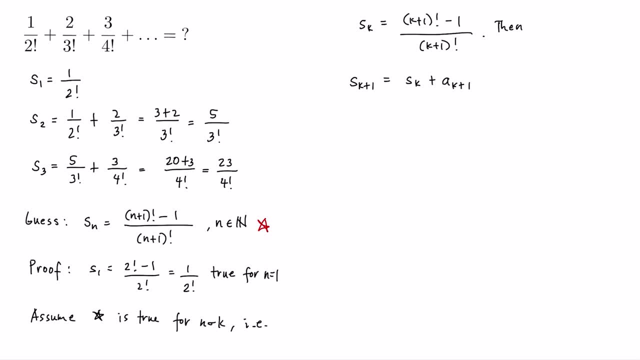 first k plus 1 terms a sub k plus 1. but in our formula, so clearly, in this case the kth term, a sub k, is equal to. you have your k over k plus 1, quantity factorial. so this is equal to s sub k. so that is k plus 1. 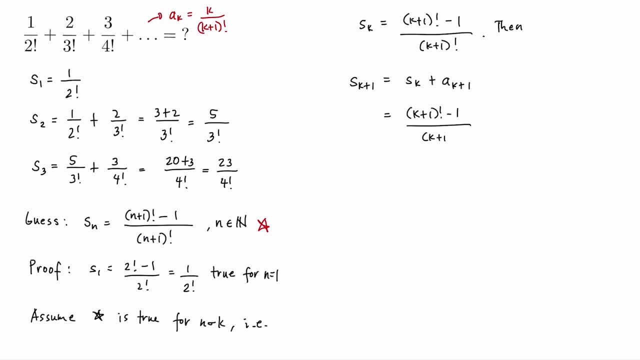 factorial minus 1, all over k plus 1 quantity factorial, and then a sub k plus 1 is equal to k plus 1 all over k plus 1 plus 1, so that is k plus 2 quantity factorial and combining this to a single fraction. so we have here k plus 2 quantity factorial and then divided by k plus 1. 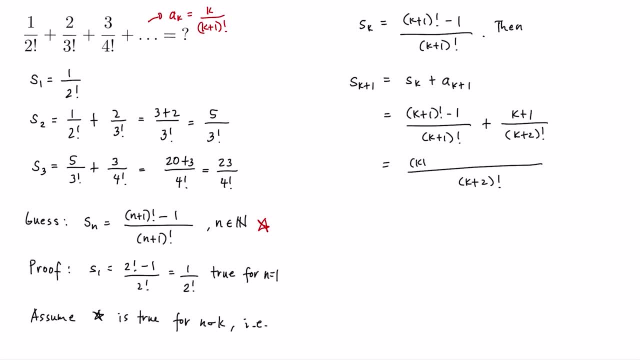 factorial. so we'll be left with k plus 2. so we have here k plus 2 times this numerator here. so that is k plus 1, quantity factorial. distribute it so minus the quantity k plus 2 and then plus the numerator of the second fraction. 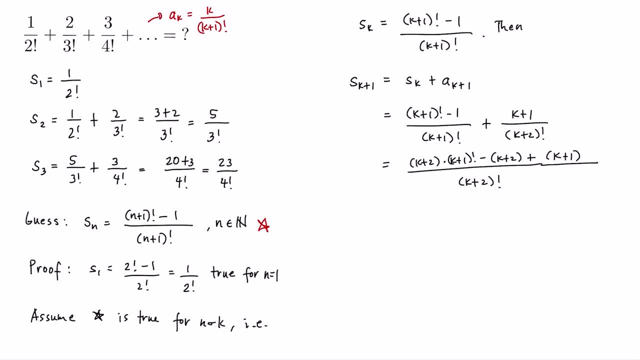 so that is k plus 1, and simplifying the numerator, we can write it as k plus 2 factorial, and then minus k minus 2 plus k plus 1, so that is minus 1 all over the quantity k plus 2 factorial. therefore our equation star is true for n equal to k plus 1 and by mathematical 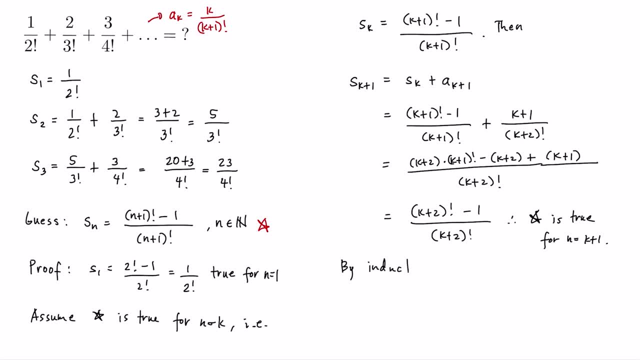 induction, so that is by induction this equation. star here holds for n element of the set of natural numbers. so now we can already find the sum of our infinite series, and the sum here is equal to the limit of this nth partial sum, s sub n, as n approaches infinity. so that is limit as n approaches. 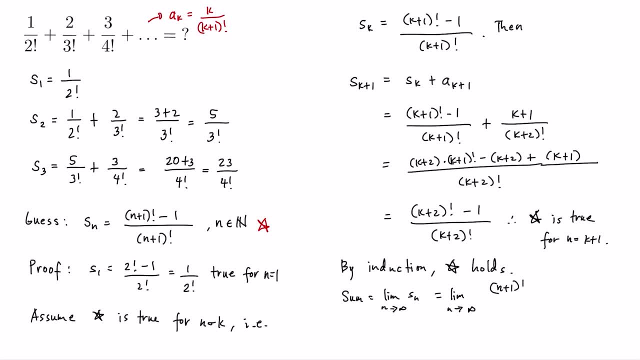 infinity of this n plus 1 quantity factorial minus 1, k plus 1 quantity factorial minus 1, over the quantity n plus 1 and then factorial, which can be written as limit as n approaches infinity of you, have there 1 minus 1 over n plus 1 quantity factorial and clearly this fraction here.